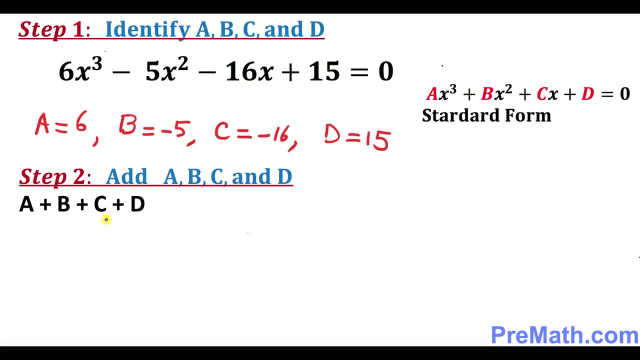 In simple terms, we want to identify our coefficients a, b, c and d. In step two, I want you to add a plus b plus c plus d and see what happens. So what happens? a is how much 6 plus b is negative, 5 plus c is negative, 16 plus d is 15.. 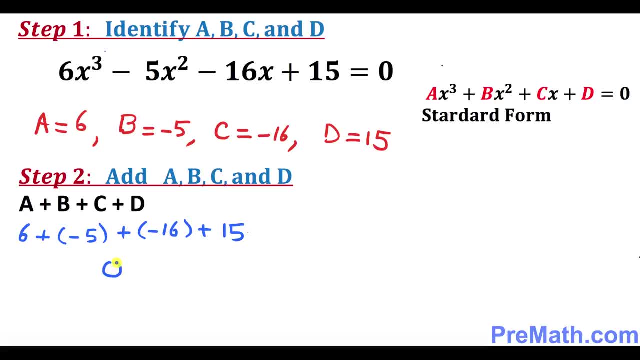 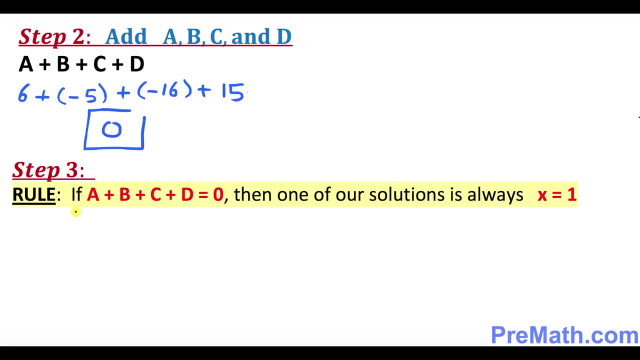 If you add them up, their sum turns out to be how much Zero. And in step three there's a very important kind of rule. This rule states that if a plus b plus c plus d turns out to be equal to zero, as in our case, 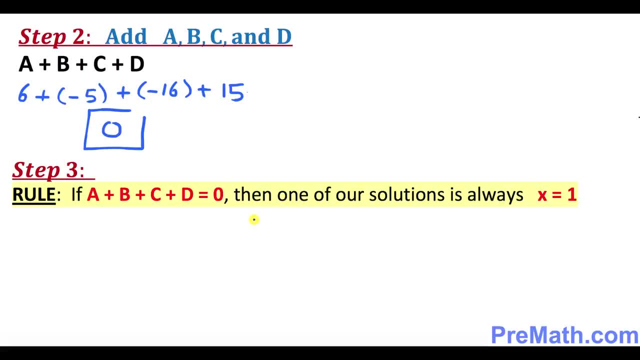 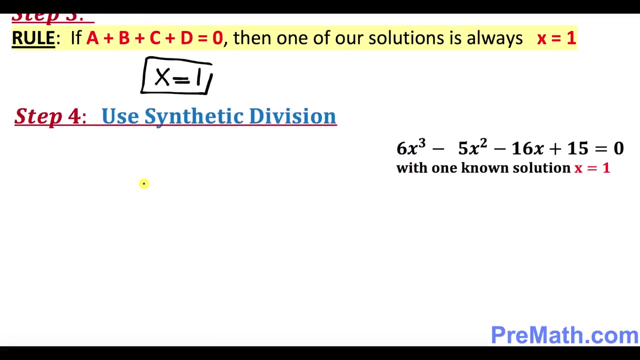 then one of our solution will always be x equal to 1 or 1.. So that means our one of the solution is what x equal to 1. Always is going to be as long as their sum turns out to be zero. And in step four, as you can see, we will be using synthetic division to figure out other solutions. 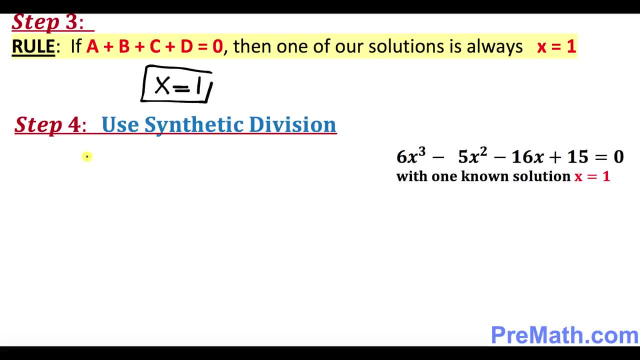 So let's go ahead and take care of the synthetic division. Okay, let's go ahead. I'm going to put down the numbers right up here. The coefficients are what? 6 negative, Negative, 5, negative, 16 and 15, right up here. 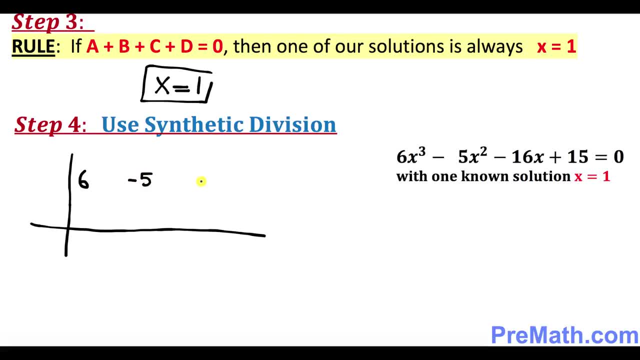 6, negative 5, negative 16, and what 15.. And, as you know that our solution, one of the solution in x equal to 1, is going to come right up here at this place, So let's go ahead and just this: 6 is going to be as it is, 6 right up here. 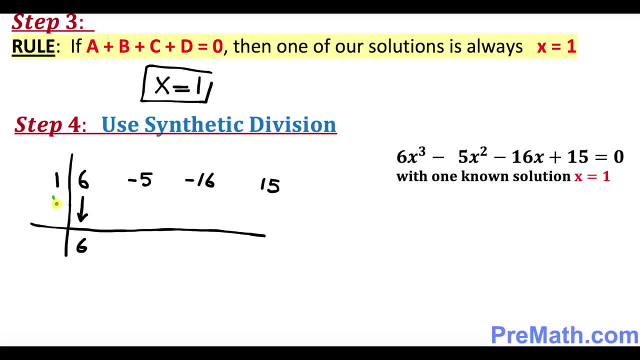 Now what we're going to do is we're going to multiply this 1 times 6 and just put it right up here. So negative 5 and 6, if you add them up, that's going to be what It's going to be: 1.. 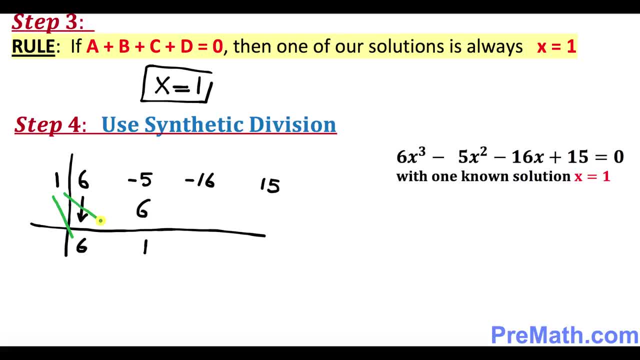 Once again, I want you to cross multiply 1 times 1.. This one that's going to give you what 1 times 1 is, what 1 negative 16 plus 1 is going to be negative 15.. Okay, 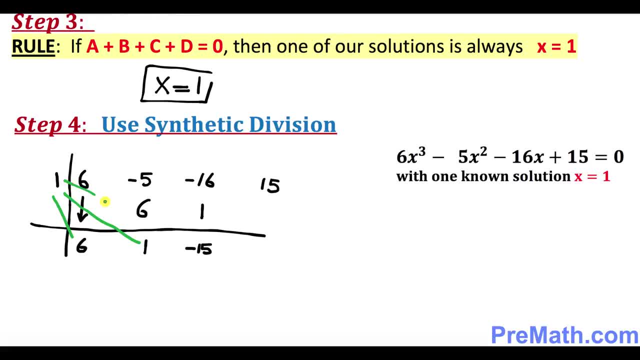 So, once again, we're going to multiply this 1 times negative 15.. And what happens? So that's going to 1 times negative. 15 is negative 15. right up here, 15 and negative 15.. When you add them, it's going to give you what. 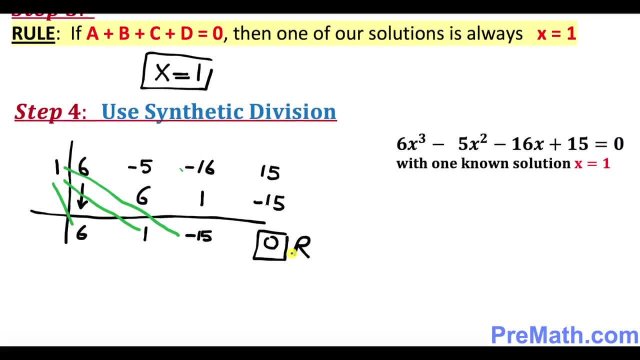 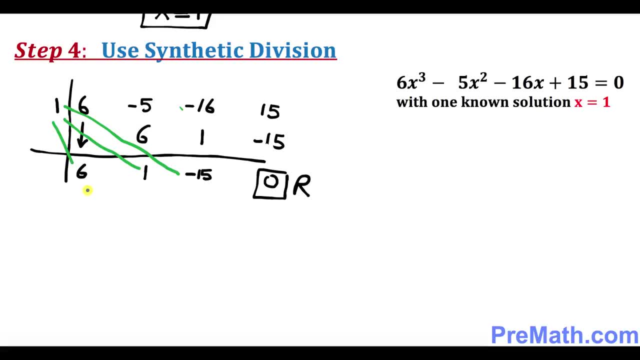 0.. That is your remainder. So we ended up with these numbers: 6, 1 and negative 15.. So now this 6 is going to be with that X, power 2, this is going to be with the X and this negative 15 is going to be without X, which is called constant. 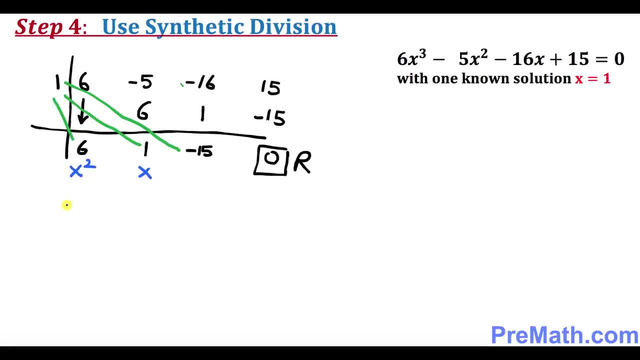 So what we got right now? so we finally got 6X squared plus 1X minus 15. equal to what? 0.. So what's going to happen right now up over here? We want to find the factors for this one. 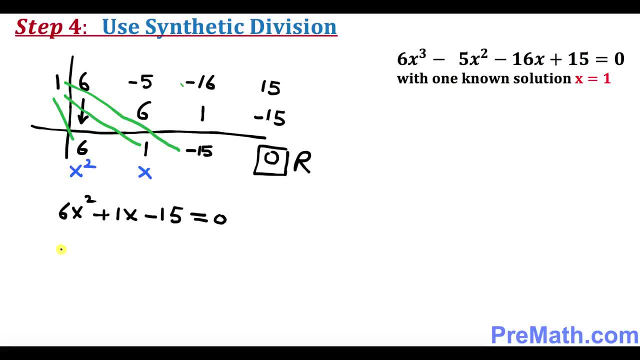 Can you figure out the factors for this one? That's going to be how much. The factor is going to be for sure is going to be what 2X minus 3, and the other factor is going to be what 3X plus 5,, which is equal to what. 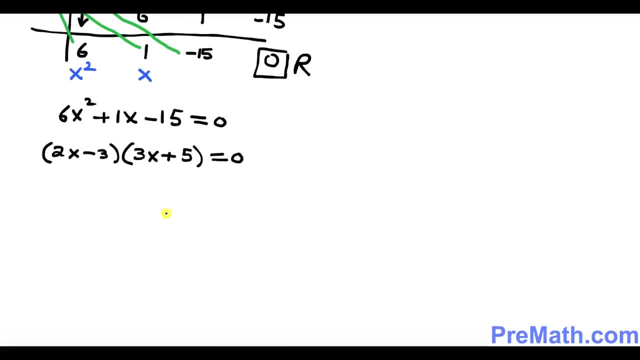 0.. All right, so since they are equal to 0, we're going to split them up. So I'm going to put down 2X minus 3, equal to 0, and the other one is going to be 3X plus 5, equal to what. 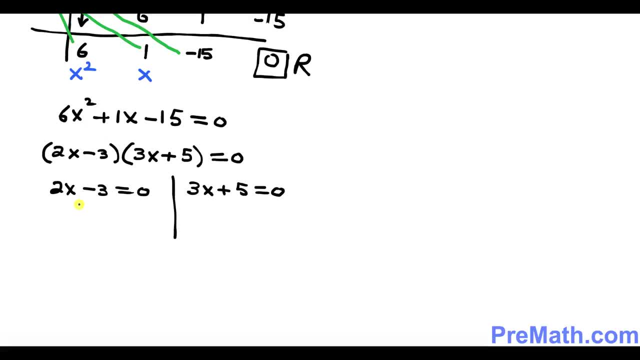 0. Let's go ahead and add 3 over here to get rid of this 3.. So if you add 3 on this side, what happens? This cancels out. So you got 2X equal to 3.. I want you to divide it by 2.. 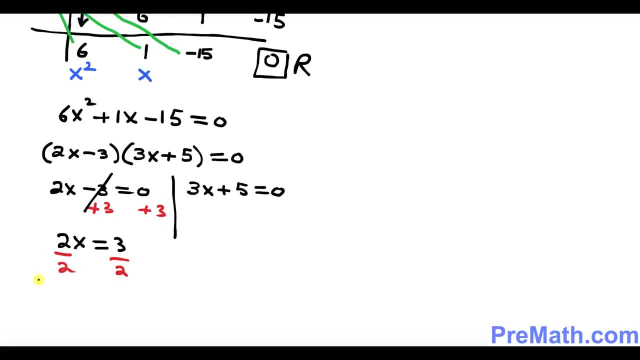 So X turns out to be 3 over what? 2.. So one of our solution is X equal to 3 over 2.. Likewise, on this side, we're going to do what We're going to subtract 5.. We're going to subtract 5 from this side. 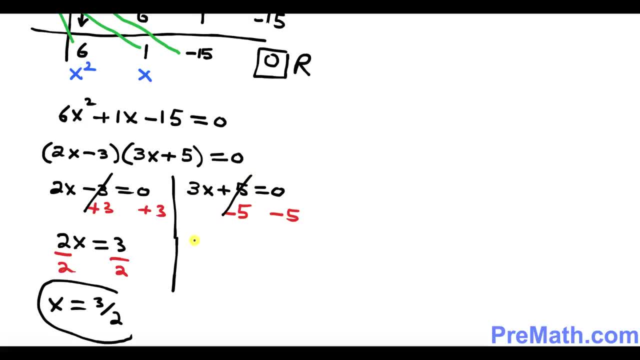 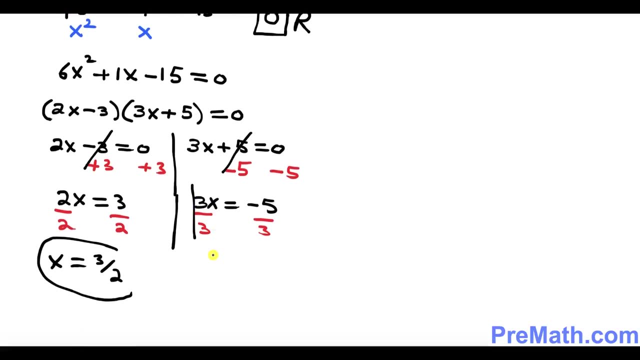 So what happens? So this thing is gone. So we got 3X, equal to negative 5.. Now I want you to divide both sides by 3.. So this, what happened? This? 3 and 3, they are gone. 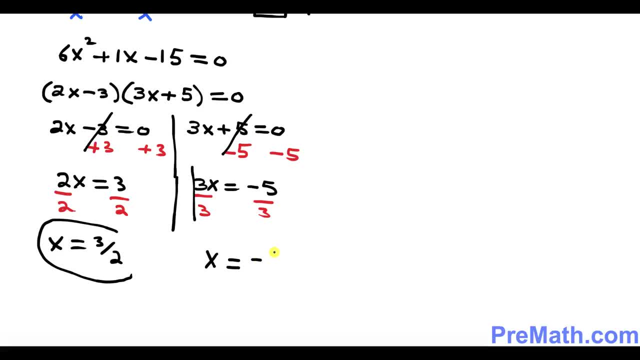 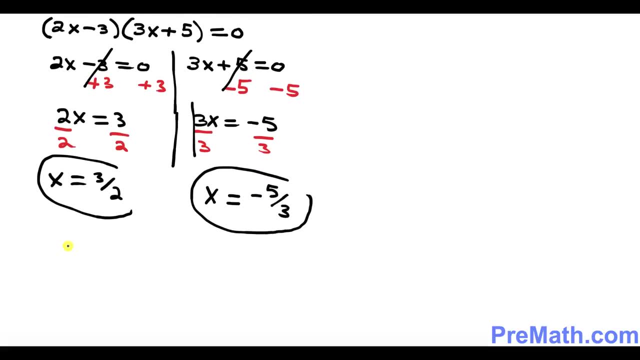 So we got X equals to how much Negative 5 over 3.. So that's your another solution. Thus, our complete solution set is going to be: simply: what So? first, we had already a solution- X equal to 1- in our previous step, as you recall. 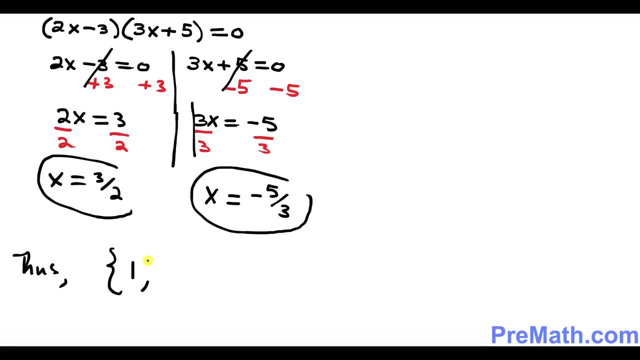 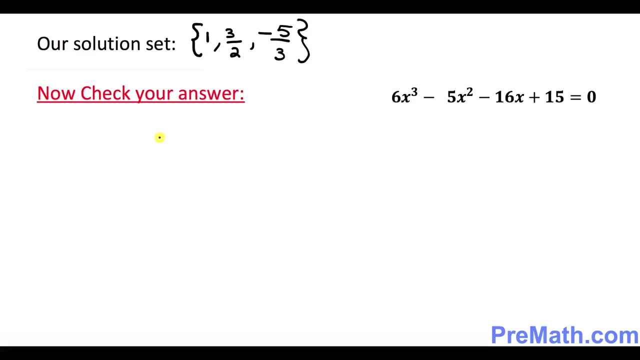 And then we're going to have what We have, what 3 over what 2.. And finally we have a negative 5 over 3 is our solution set, So we have 4 over 3.. And then finally, in our this step, we want to check our solution, our answer. 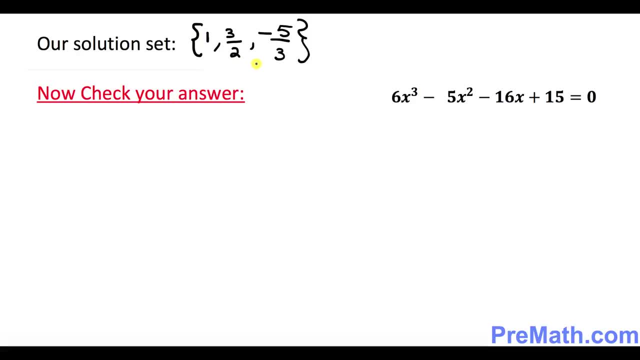 So, the very first thing, what I want you to do is go ahead and whatever your solutions are, you just add them up. I'm going to put down 1 plus 3 over 2, plus negative negative 5 over 3 and ask yourself: is it equal to negative b over a? and now you might be wondering: 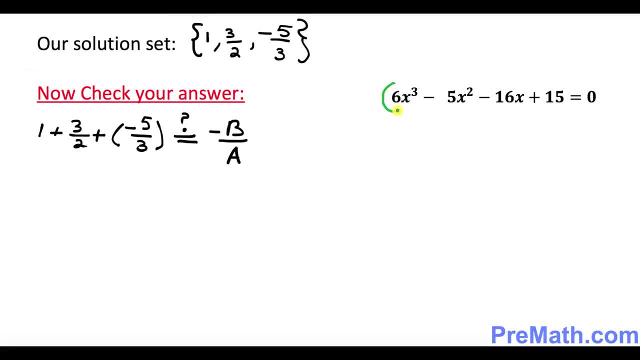 what is negative, b over a? In our case, a equals to 6, b equal to negative 5, c equal to negative 16 and d equals to 15.. So minus b over a is going to be simply what negative and negative 5 over what?